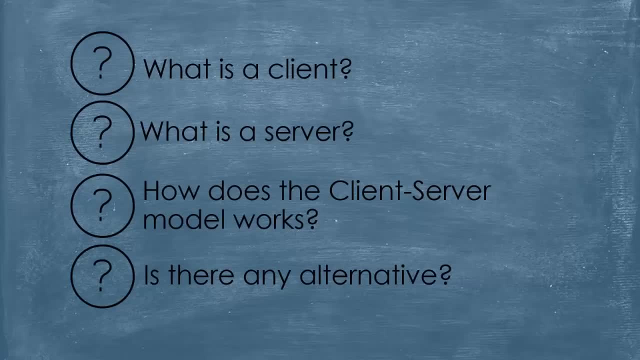 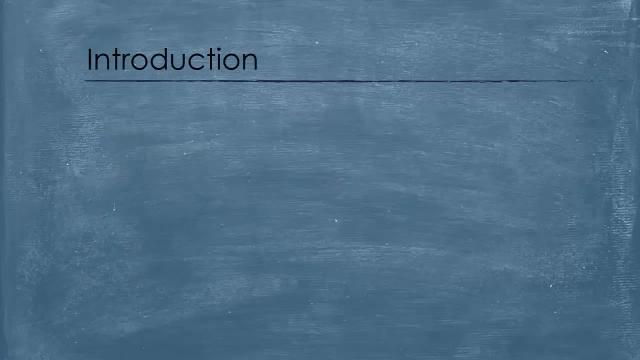 works, and is there any alternative to that? We will answer all these questions and more Well, what are we waiting for? Let's dive in. Let's begin with a brief introduction. The web is a service which is built on top of the internet to allow computers 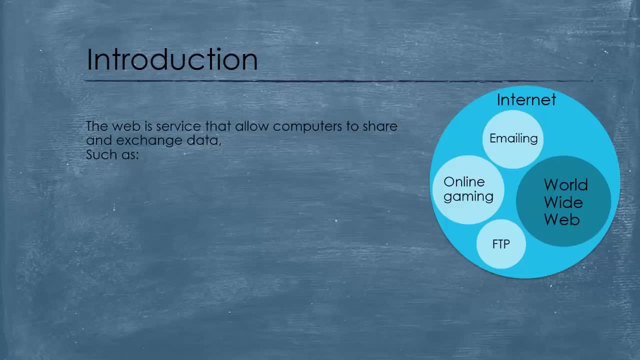 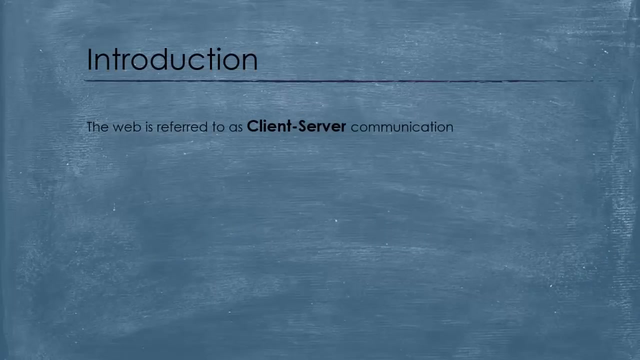 to share and exchange data easily and reliably. And when we say data, it can be anything such as images, videos, documents, etc. in any form, And for that sometimes the web is referred to as a client-server model communication, because there are always 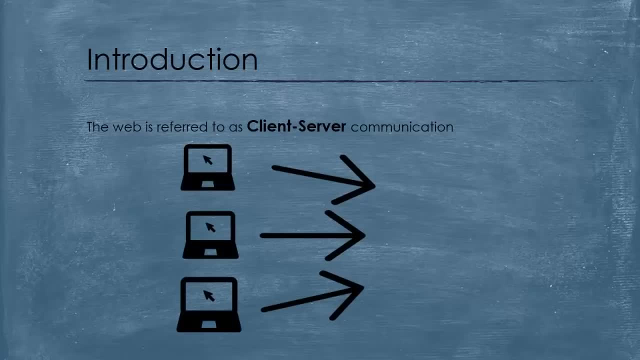 computers that ask for data, which are called clients, And the computer that gives the data, in other words, the computer that provides the data. Thank you for watching and see you in the next video, Bye-bye. computer that serves, which is the server? now let's be more specific. what is a? 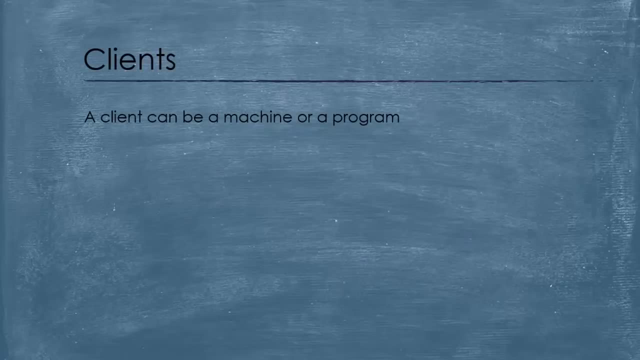 client. a client can be a machine or a program. when we say a client machine, we are actually talking about the devices that the end user can use to access the web. for example, your laptop or desktop is a client. smartphones, tablets, etc. are all clients machines. on the other hand, a client program is a program that allows. 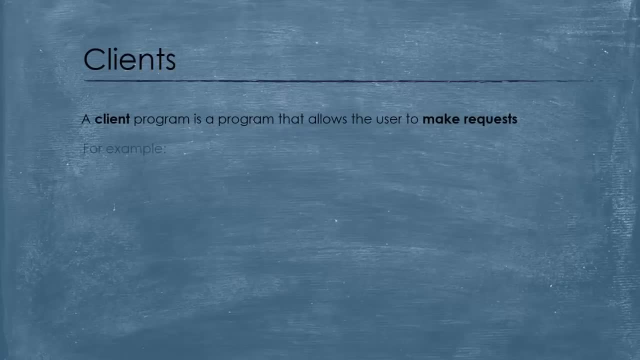 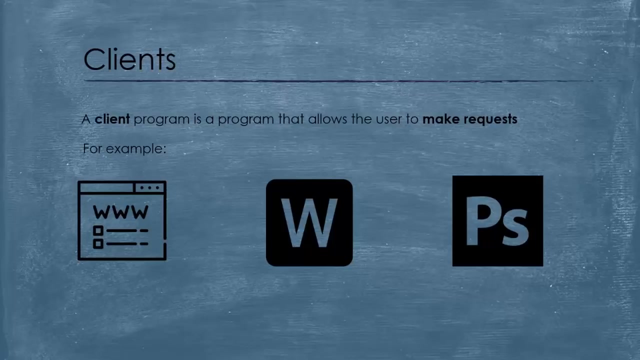 the user to make requests through the web. can you think of one? yeah, a web browser is a client program. a user can make a request for a web page through the web browser, right? can you think of another one? some programs such as word processors or photo editing software have an excess of online resources that. 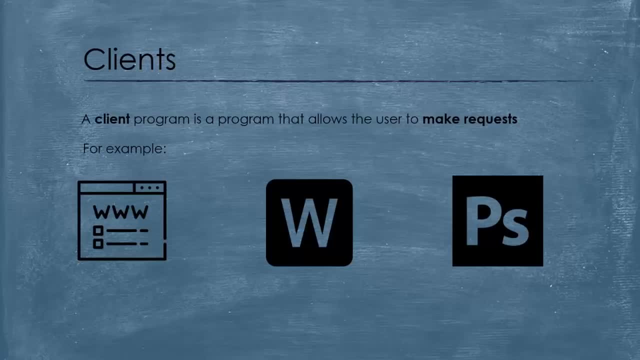 you can get from their servers, such as themes or I don't know, maybe help. sometimes you find online support. in this case, these programs are called clients, so what you need to remember is that a client, whether it is a machine or a program, is an appliance. you need to remember is that a client, whether it is a machine or a program, is an appliance, and 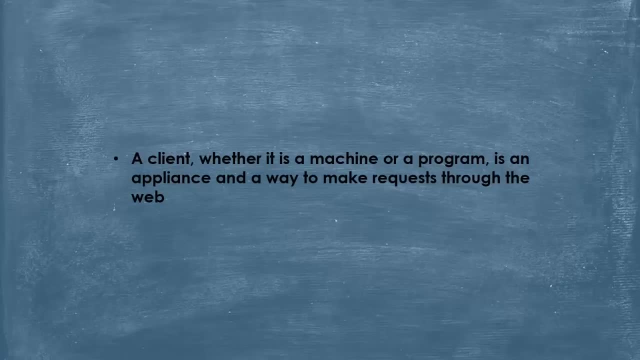 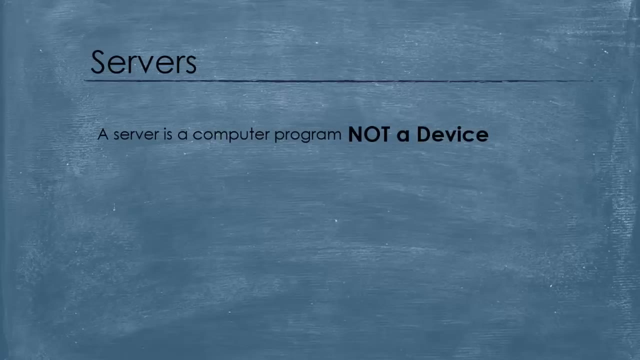 a way to make requests through the web. okay, this is what we mean by a client. a server on the other side is a computer program, not a device. a computer program. here we want to understand and clarify everything. okay, because we see people define servers as high-performance computers. yes, those computers are. 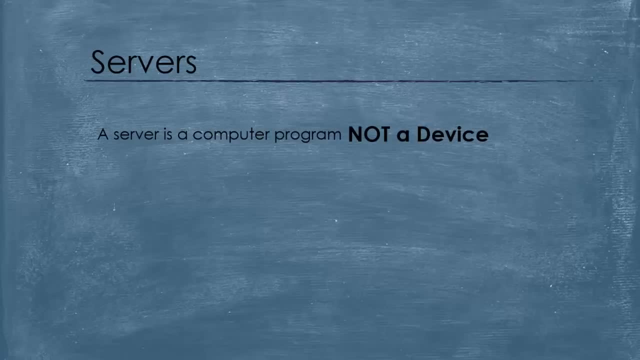 servers in some extent, but strictly speaking they are called so because they run programs that serve requests. they run server programs that provide functionality and serve other programs called clients, and also because they run server operating systems. we can run a Windows 10 or a Linux desktop version on a high-performance machine, right, so they. 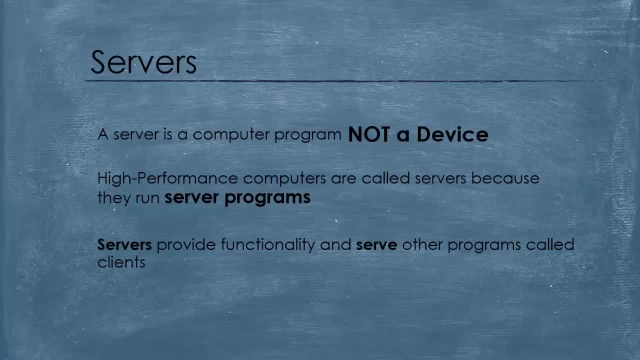 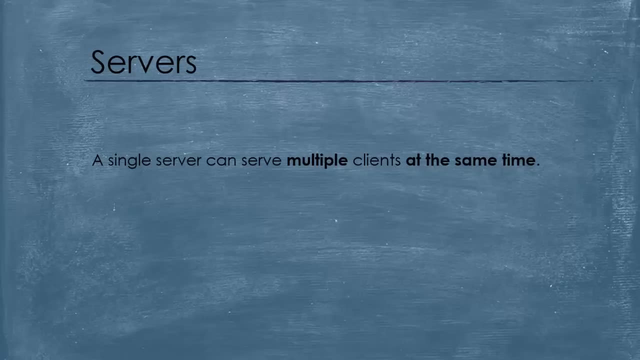 are called servers because they run server programs. a single server can serve multiple clients at the same time, and it runs 24: 7 without stopping. this is why we need actually supercomputers to run such programs also. we can run multiple servers on a one single machine, and here we are. 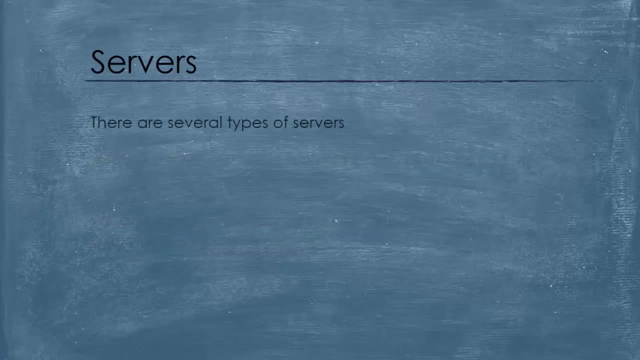 talking about virtual servers. there are several types of servers. each one serves by doing a specific task. for example, web servers such as Apache serve HTTP requests, database servers run a database management system, such as my sequel, and other types of servers. I will talk about them in detail in another video. now we 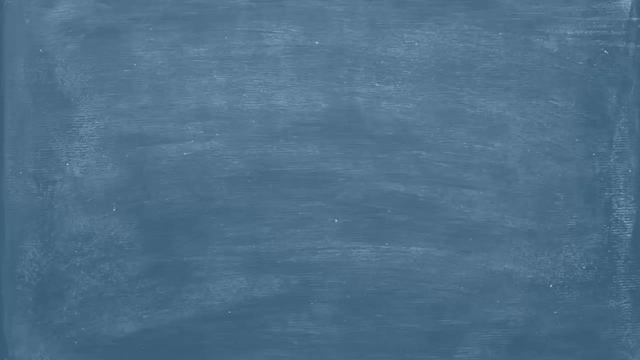 can stay here all the day talking about servers and how to run servers in a virtual machine, and we talked about servers and their types and how they work, but here's what you need to know. a server can contain web resources, host web applications, source user and program data and do a lot of things, and it is 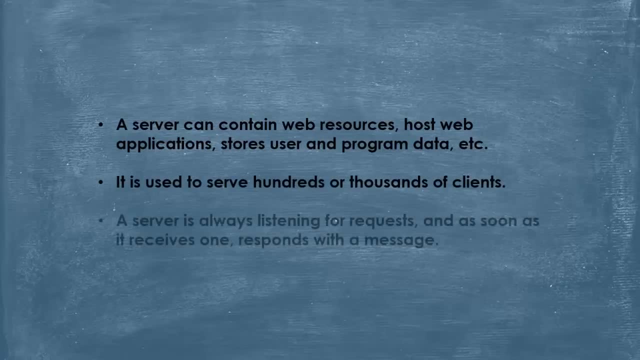 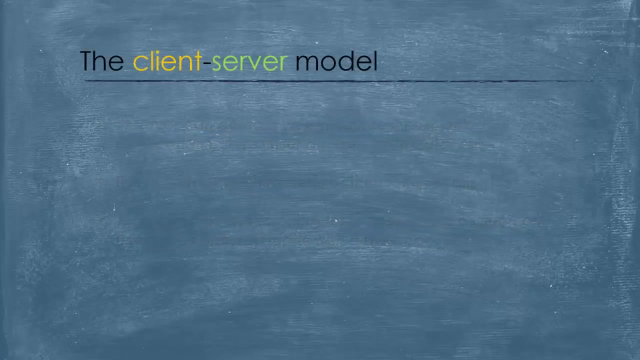 used to serve hundreds or thousands of clients. also, a server is always listening for requests, and as soon as it receives one, it responds with a message. now that we know what exactly a client in a server is, we can define the client server model sentence. the client-server model is an architecture on the web that splits computers into two sections. 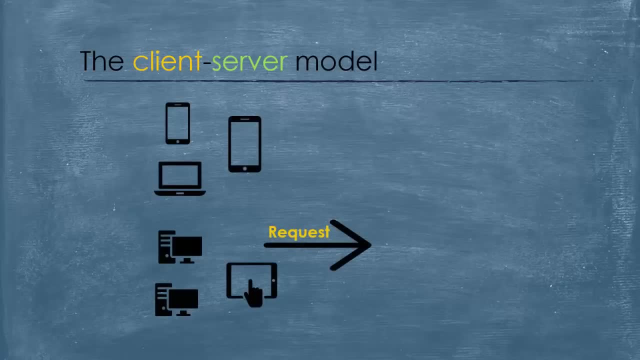 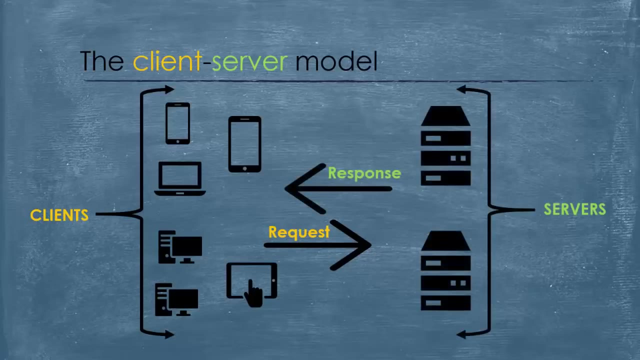 computers that ask for and request services, and they are called clients, and computers that serve clients, and they are called servers. the client-server model works through request response cycle via http messages- and to explain that i need another five minutes, which is why i dedicated a whole video to that- the http and the web. it's also worth mentioning that the client-server